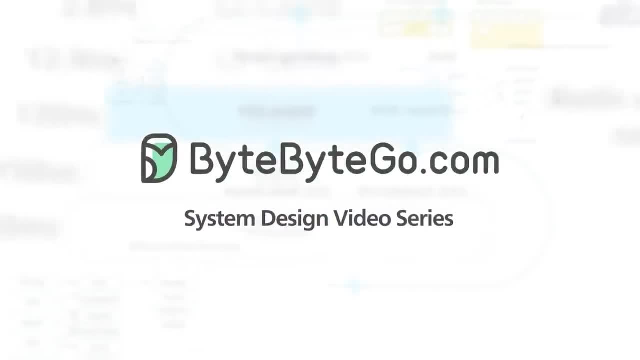 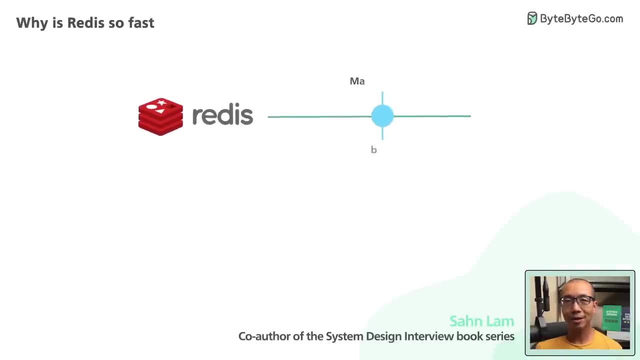 Why is Redis so fast? What fundamental design decisions did the developers make more than a decade ago that stood the test of time? Let's take a look. Redis is a very popular in-memory database. It's rock solid, easy to use and fast. These 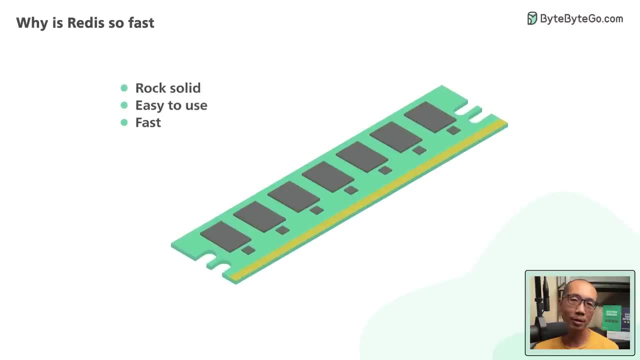 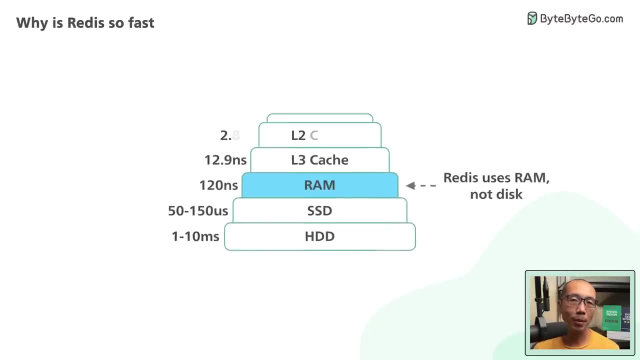 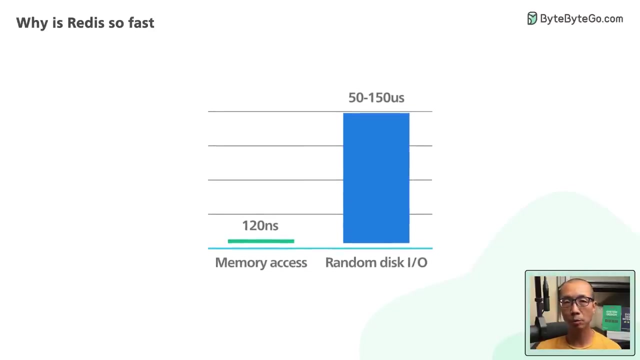 attributes explain why it is one of the most loved databases, according to the Stack Overflow's annual developer survey. The first reason Redis is fast is because it is an in-memory database. Memory access is several orders of magnitude faster than random disk I-O. Pure memory access provides high read and write throughput and load latency. The trade-off is 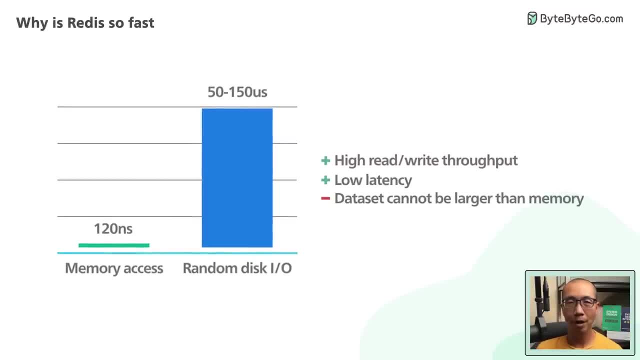 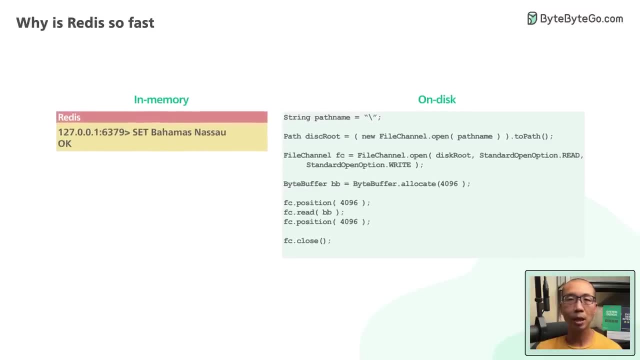 that the data set cannot be larger than memory. Code-wise in-memory data structures are also much easier to implement than their on-disk counterparts. This keeps the code simple and it contributes to Redis' rock-solid stability. Another reason Redis is fast is a bit unintuitive. It is primarily single-threaded. 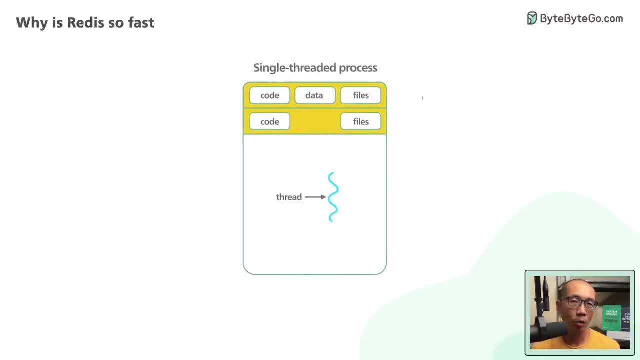 Why would a single-threaded design lead to high performance? Wouldn't it be faster if it uses thread to leverage all the CPU cores? Multi-threaded applications require locks or other synchronization mechanisms. They are notoriously hard to reason about. In many applications. the added complexity is bug-prone and sacrifices stability. 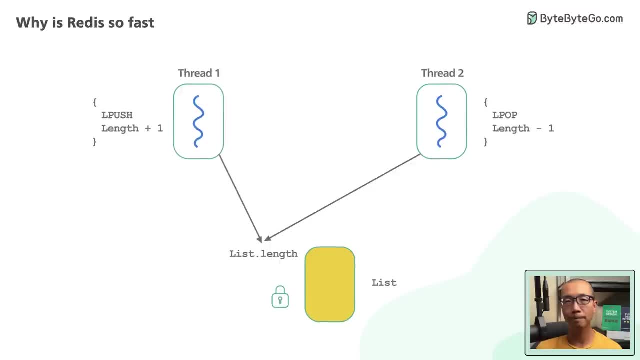 making it difficult to justify the performance gain. In the case of Redis, the single-threaded code path is easy to understand. How does a single-threaded codebase handle many thousands of incoming requests and outgoing responses at the same time? Won't the thread get blocked? 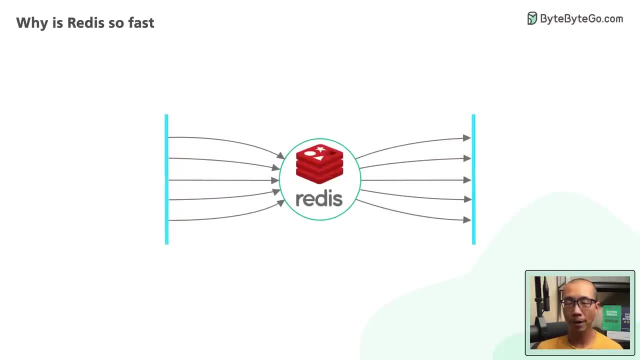 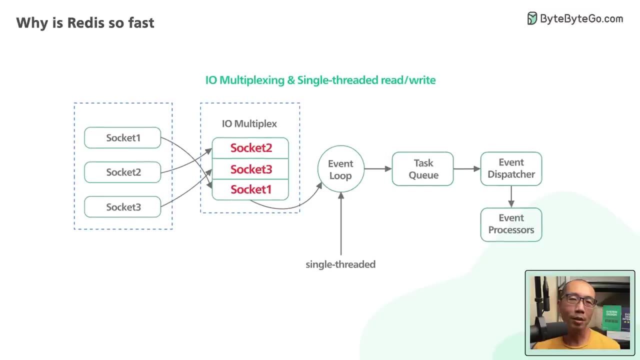 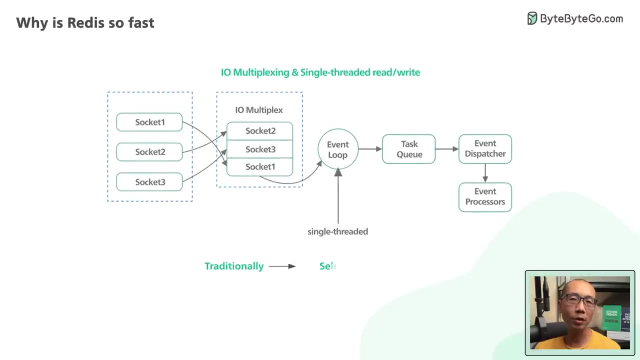 waiting for the completion of each request individually. This is where I-O might be helpful. I-O multiplexing comes into the picture. With I-O multiplexing, the operating system allows a single thread to weigh on many socket connections simultaneously. Traditionally, this is done with the select.